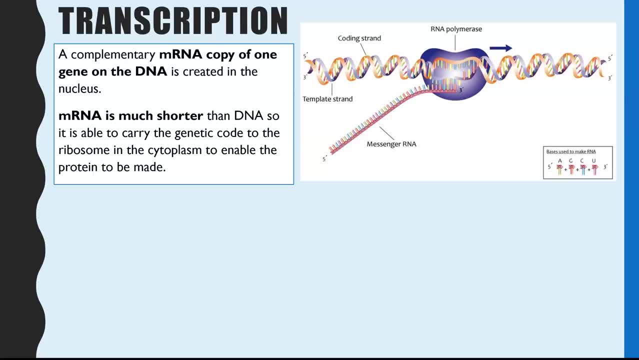 cytoplasm, there are enzymes which could damage the DNA. So instead we make a copy of the gene of interest and that copy is made in the form of messenger RNA. Now, because this is only a copy of one of the genes on DNA, and humans have approximately 23,000- 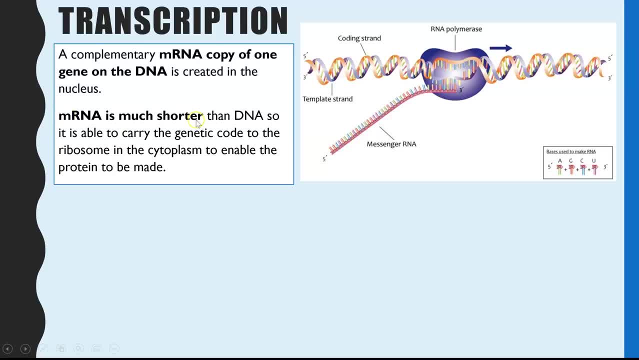 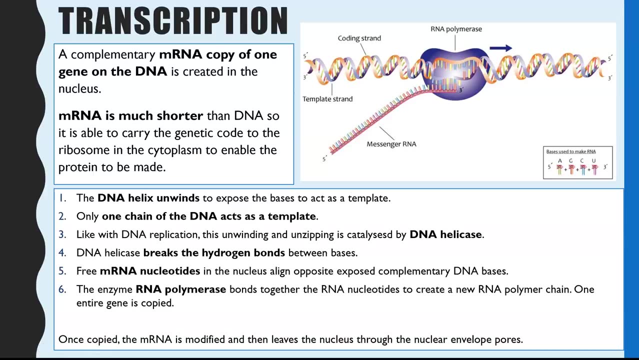 genes. it is a much shorter molecule than DNA and that is why it is actually small enough to fit through the nuclear pores, in the nuclear envelope, and therefore it can move into the cytoplasm and attach to ribosomes. So the actual process, then, and I've put all of the key marking points. 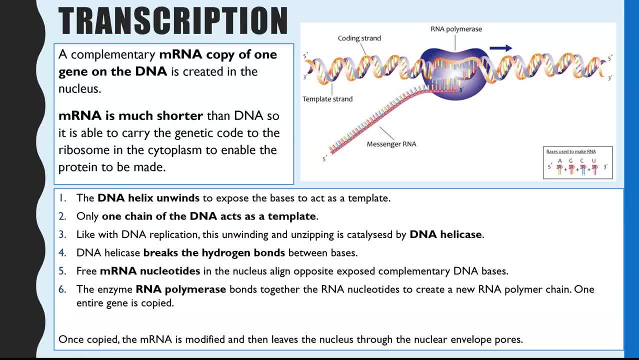 for this in bold, so you know what are the key terms you would have to include in a long answer. question about transcription. So, step one, we have to get the DNA double helix to unwind and expose the two strands, and that is because one of those DNA chains will act as a template to make mRNA and 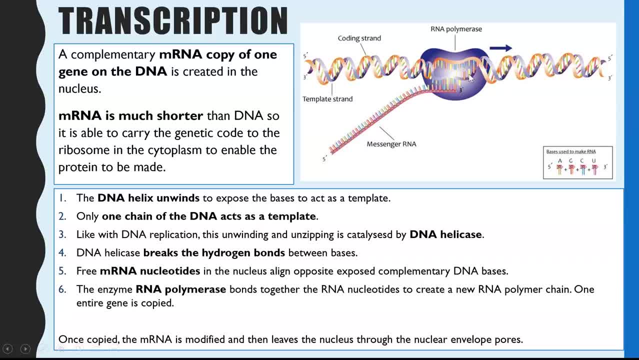 it is only one of the DNA strands this time, compared to DNA replication, That acts as a strand, because mRNA is single-stranded. Now, to do this- it is very similar to DNA replication- in order to unwind that double helix and break the hydrogen bonds between the bases of these two. 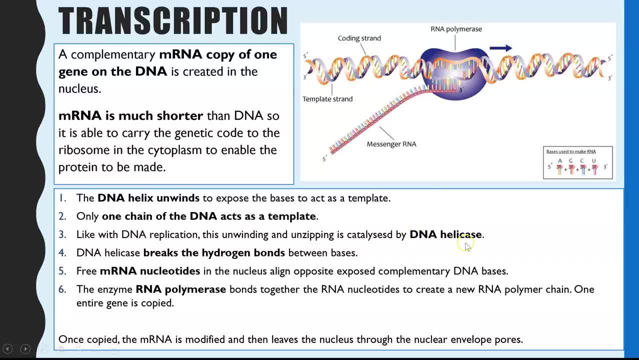 chains of DNA. the enzyme DNA helicase is used so that breaks the hydrogen bonds. So we now have one of those strands exposed, ready to be the template You'll then have. within the nucleus there are free floating RNA nucleotides and we can 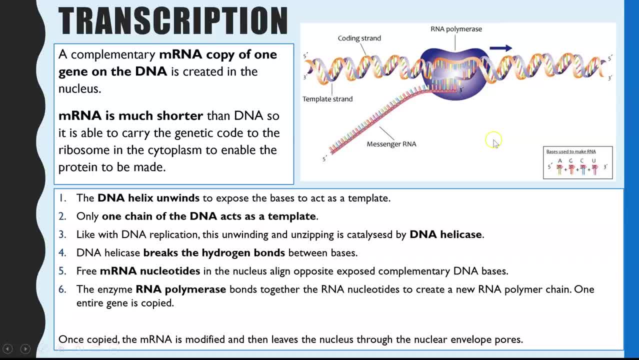 see the four options of those down here. Now, if they happen to align opposite their complementary base pair on this exposed strand, they'll be able to stay in that position and then RNA polymerase will join all of those nucleotides together by phosphate diester bonds. This is all through the 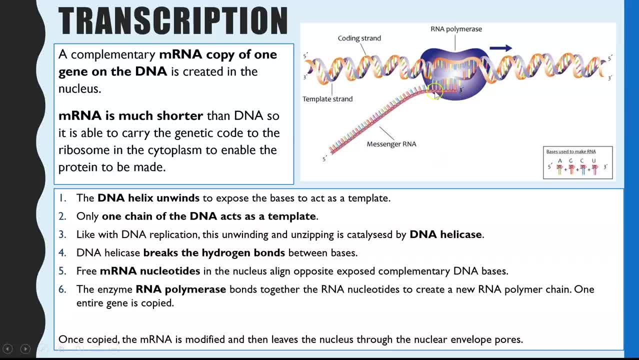 idea of complementary binaries, base pairing again. so the dna bases, the rna bases which are complementary to those, will align opposite. so you've then got your entire copy of mrna, and at this stage we actually call it pre mrna, and that's because it has to be modified before it leaves the nucleus. so those modifications, 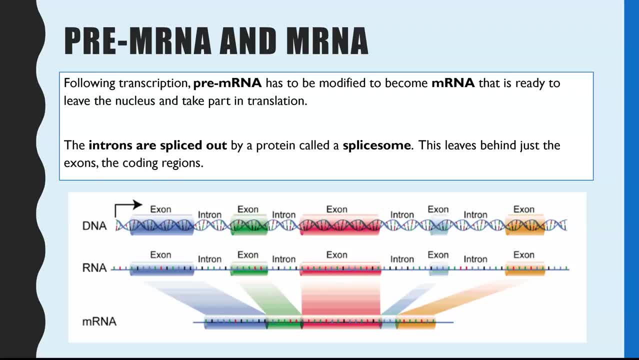 the main modification and the one that you need to learn about for aqa a level is what we call splicing, and that is when we remove the introns. so our dna is approximately 98 introns, and introns are the sequences of bases in your dna which do not code for amino acids. 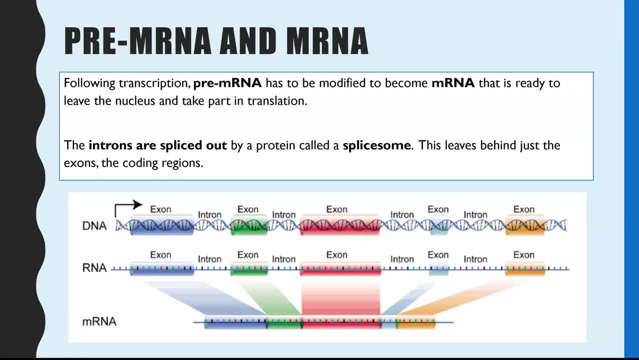 and therefore we have to remove them from the mrna before it goes away, and that's what we call splicing, because we actually need to remove the microclimates and this goes to the ribosome, and these introns are removed by a splice zone, which is a protein. 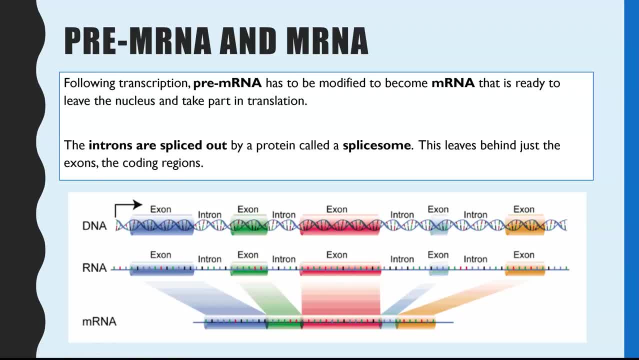 which can attach to the dna cut and break those phosphine diester bonds and therefore it cuts out the introns. however, because this is done by a splice zone, we actually describe that as splicing rather than cutting. so the introns have been spliced out and you would have to use that. 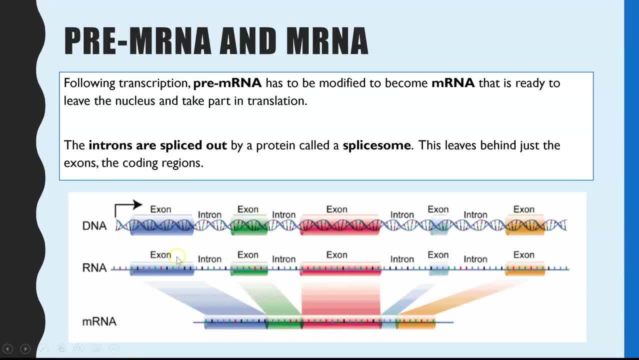 terminology, rather than saying: this is just a splicing. but we can also use splicing as a way to saying they've been cut out, so they get spliced out and removed. so that then means your finished mRNA is just made up of exons, which are just the coding regions of the DNA. Now I did actually talk. 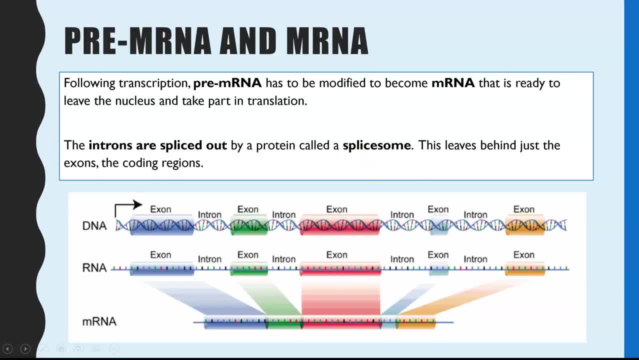 about introns and exons in my genetic code video, which I'll link here so you can watch. You might be wondering why do we have 98% of our DNA as introns if it's described as junk DNA? it doesn't code for anything and it gets cut out. The answer to that isn't actually on the AQA specification. 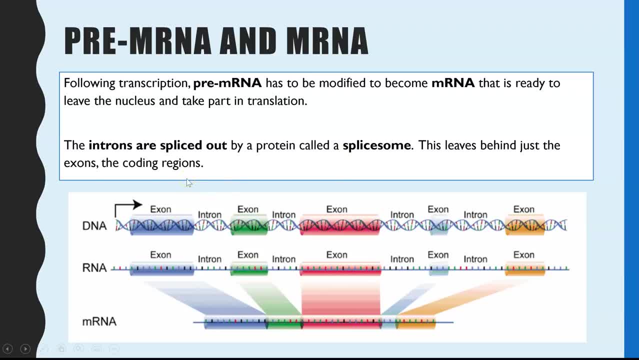 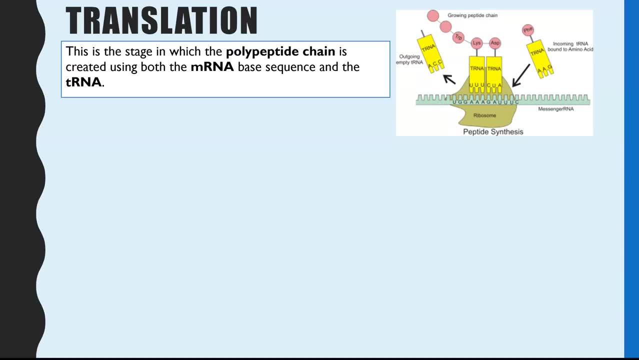 so I'm not going to go through it. however, if you are interested, research alternative splicing. So the next step and the final step is translation. So this is the stage where the polypeptide chain gets created, which is that primary sequence of a protein, the primary structure, the sequence of 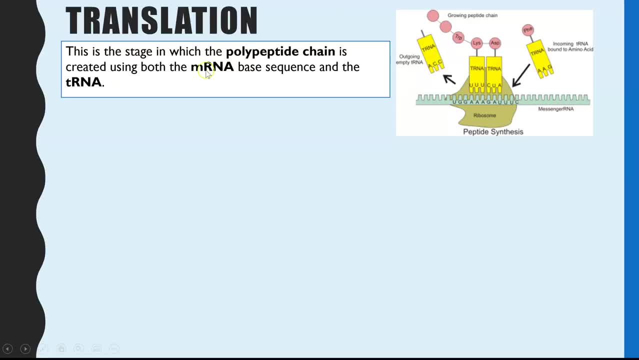 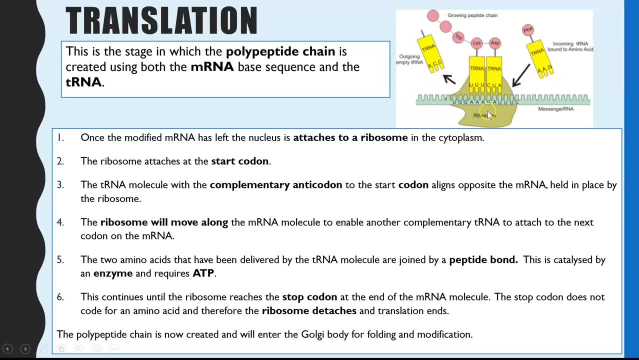 amino acids, and this is created using mRNA and tRNA, and this is within the cytoplasm, with the mRNA attached to the ribosome. So that's the first step. once that modified mRNA leaves the nucleus, it then attaches to a ribosome, at the start codon and the start codon is the first three DNA or, in this case, mRNA bases. 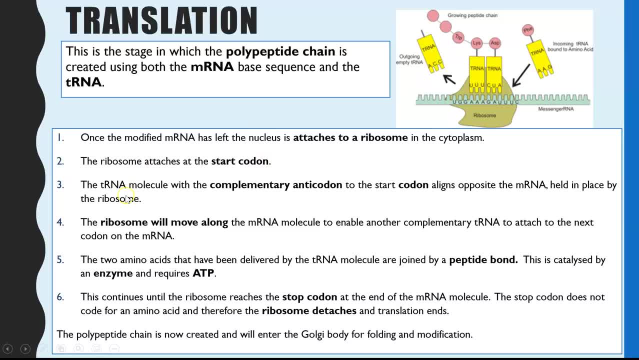 at the start of the sequence, And these are tRNA molecules that are just floating around within the cytoplasm. Each tRNA molecule has an anticodon, which is three bases at its bottom and an amino acid attachment site at the top, And therefore each tRNA molecule will bring a specific amino acid determined by the anticodon and therefore the codon on mRNA. 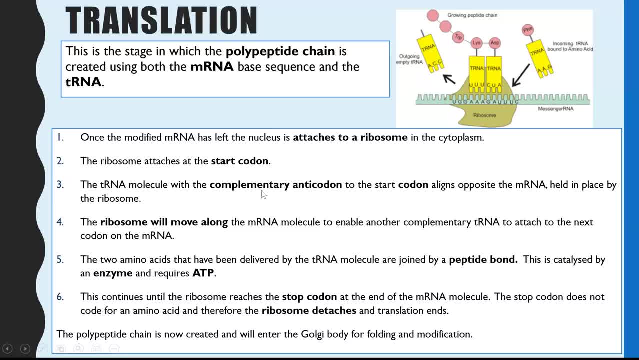 So the tRNA molecule with the complementary anticodon to the start, codon, which is our first codon on the mRNA, will align opposite the mRNA and the ribosome holds them in place. So that's the role of the ribosome: It holds the mRNA and tRNA in place. 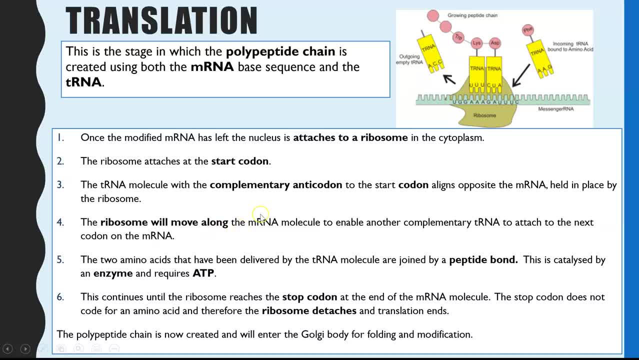 The ribosome will then move along and the mRNA codon, which matches the tRNA matches to a different, potentially complementary tRNA anticodon, will then align, And the ribosome can hold about two tRNA molecules at a time. 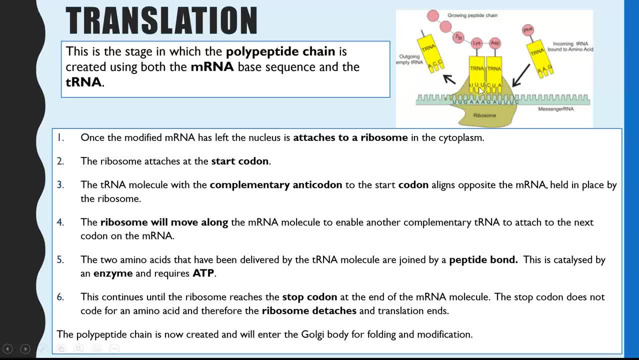 So we now can see, we've got two tRNA molecules here. They are aligned opposite the complementary codon to their anticodon, And while the ribosome holds them in place, what then happens is the two amino acids at the top, at the top of the tRNA molecule. 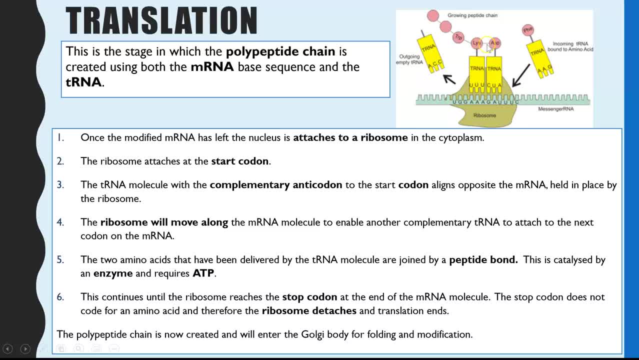 join together And this is where the peptide bond is created. Now, to create that peptide bond, there has to be an enzyme And it also requires ATP. So this is why protein synthesis requires energy. It's because to make that peptide bond between amino acids,